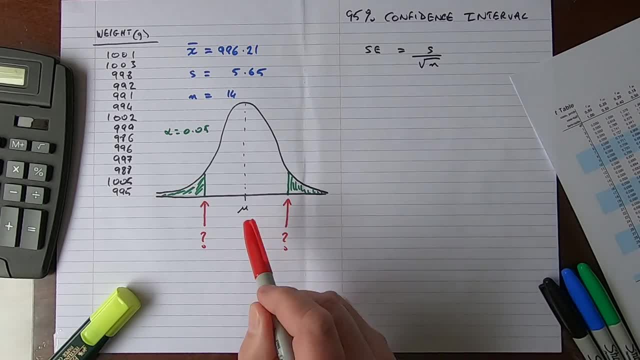 our friend the bell-shaped diagram here. and what we say for 95% confidence is that if it's bell-shaped like this, with the population mean mu in the center, here 95% of all values fall between this area, here the vast majority of the bell shape and 5% fall into the left and the right tail, so half. 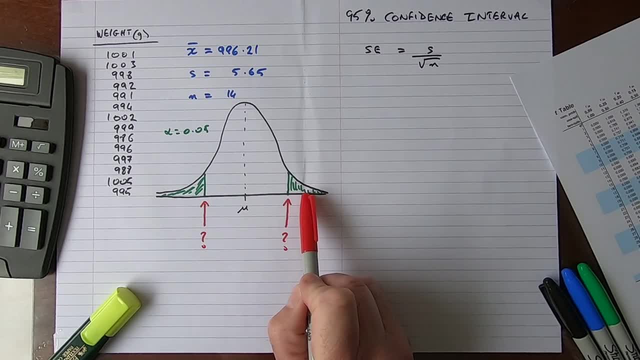 of 5% in the left tail and half of 5% in the right tail. So what we need to know here for our sample size is: what is the value? what is the t value here, at each of these margins, at each of the tails? 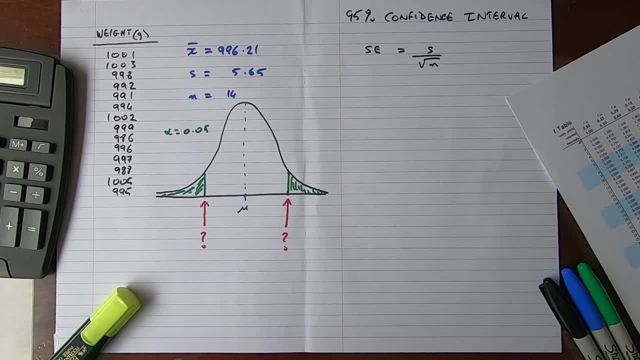 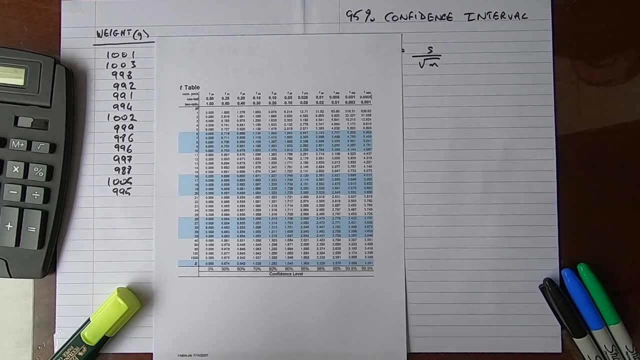 So we're going to need to look those up in t tables, So let's go ahead and do that first. So these are t tables here and they're widely available online. and there's two things we need to know. We need to know down the left hand side here. 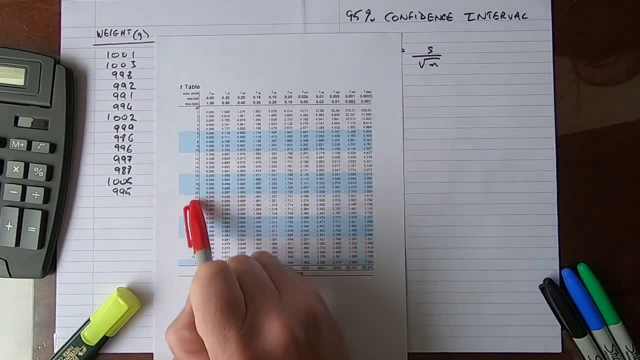 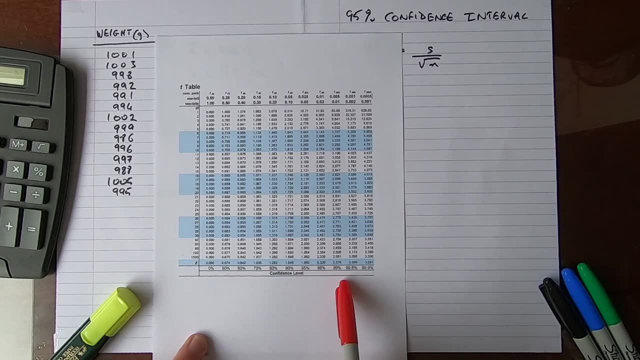 what the row is, and that's based on df degrees of freedom. So we're going to need to have to work out the degrees of freedom for our sample size of 14 and we also then need to know what level that we want to do our test that. so we're doing it at 95 percent here, or a value of 0.05. 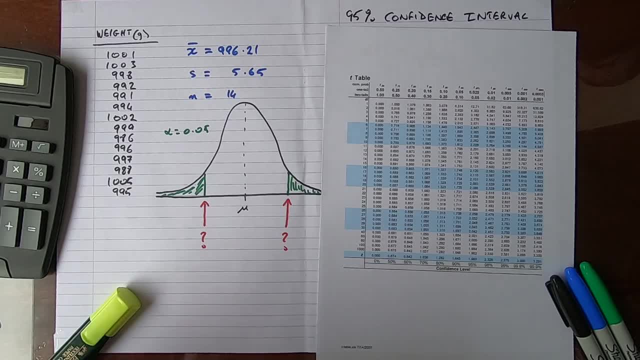 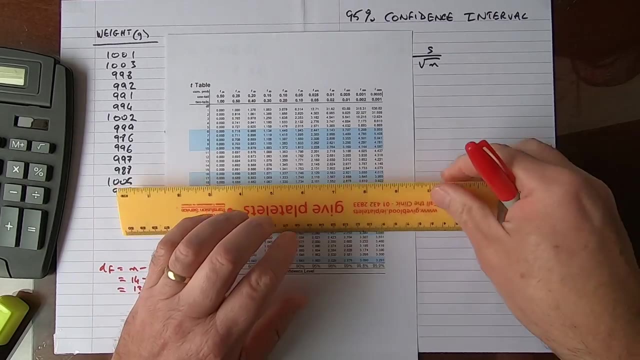 so the degrees of freedom, first of all, are straightforward enough, and the degrees of freedom is equal to n minus 1, which is equal to, in our case, 14 minus 1, which is equal to 13. so we have 13 degrees of freedom. so let me go and look this up on the table. so on my row here of 13. so 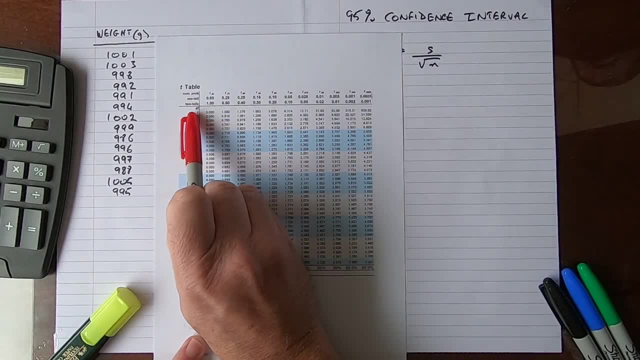 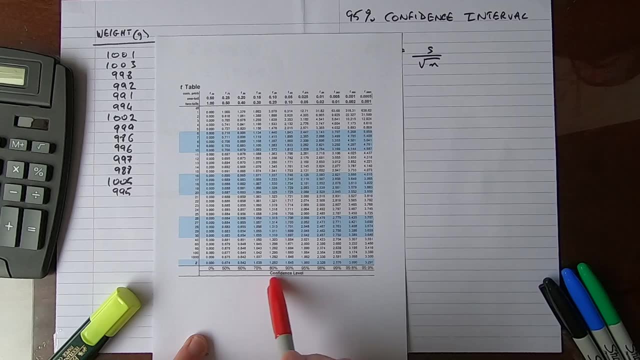 know down the left hand side here what the row is, and that's based on df degrees of freedom. So we're going to need to have to work out the degrees of freedom for our sample size of 14, and we also then need to know what. what is the confidence level of the sample size? So we're going to need to know. 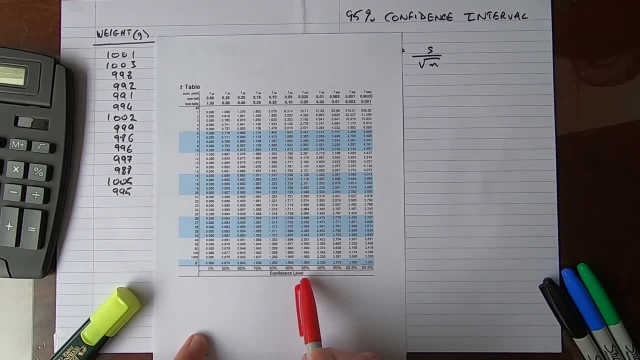 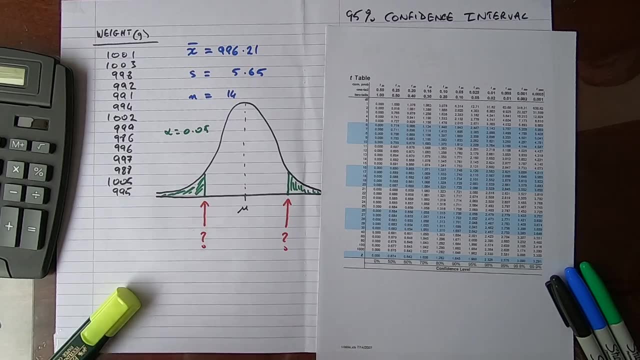 the confidence level that we want to do our test, that. So we're doing it at 95% here, or a value of 0.05.. So the degrees of freedom, first of all, are straightforward enough, and the degrees of freedom is equal to n minus 1, which is equal to, in our case, 14 minus 1, which is equal to 13.. So we have 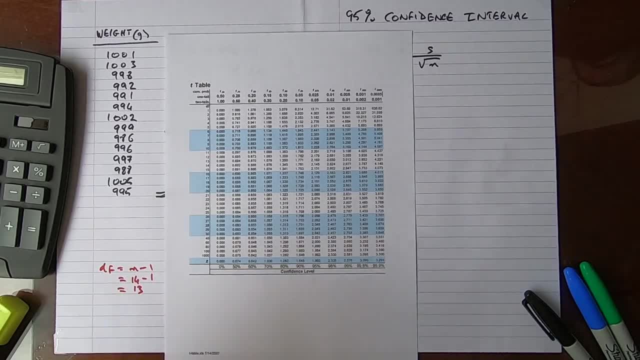 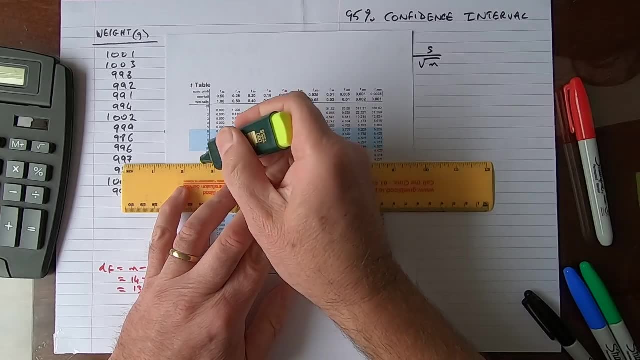 13 degrees of freedom. So let me go and look this up on the table, So on my row here of 13, so somewhere on this row, if I just highlight the row, somewhere on this row is my t-value. Now, how do I select the column? Well, 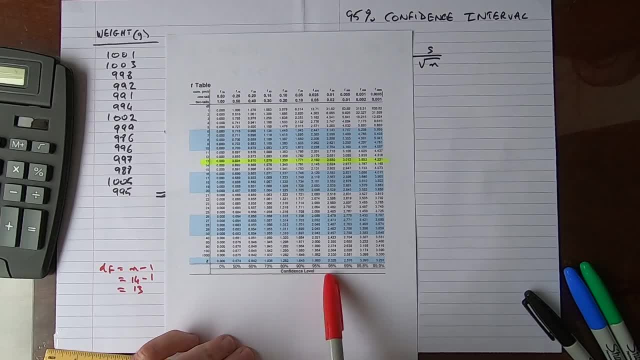 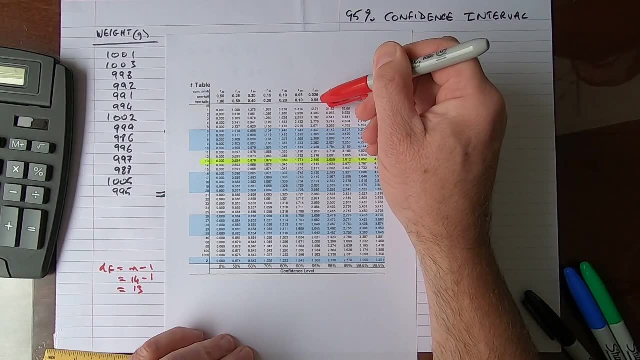 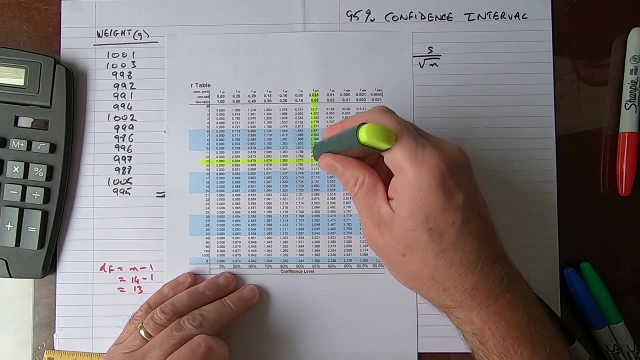 the column is. I can do it in two ways. One is I can cross the bottom in this version of a t-table. look and see 95% here. so that will be in this column or at the top. I can choose. we've got two tails, the value of 0.05.. So somewhere on this column is going to be my t-value and where the 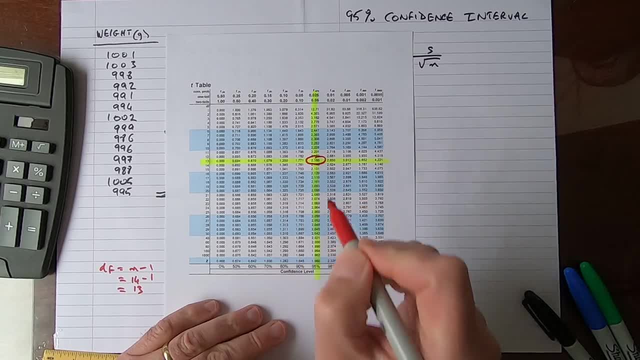 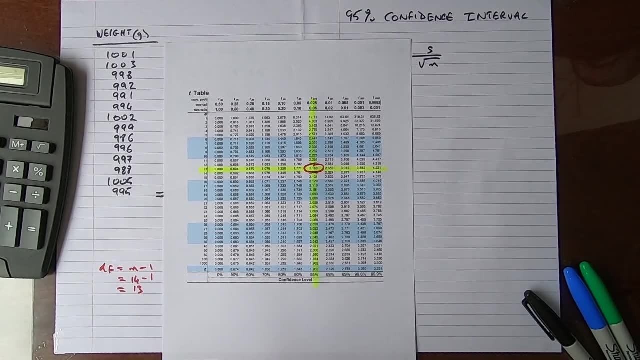 two values cross over is the t-value. So I can do it in two ways. So I can do it in two ways. So basically I have the 3 and the t value I'm going to need. We can see that that is 2.160.. 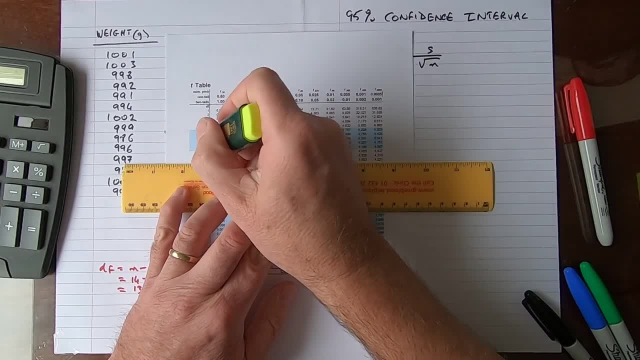 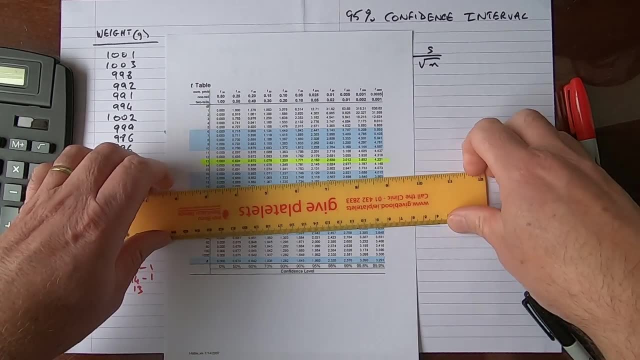 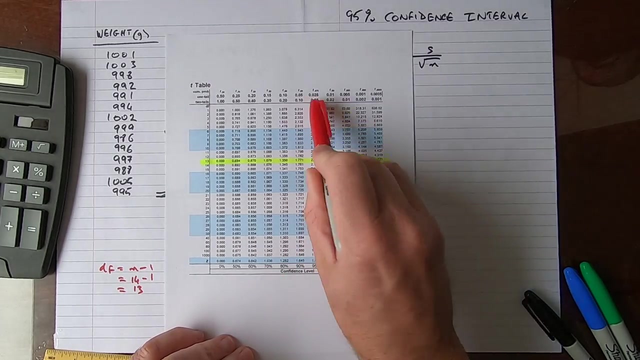 somewhere on this row. if i just highlight the row, somewhere on this row is my t value. now how do i select the column? well, the column is: i can do it in two ways. one is: i can cross the bottom in this version of a t-tab- look and see 95 here- so that will be in this column or at the top. i can choose. 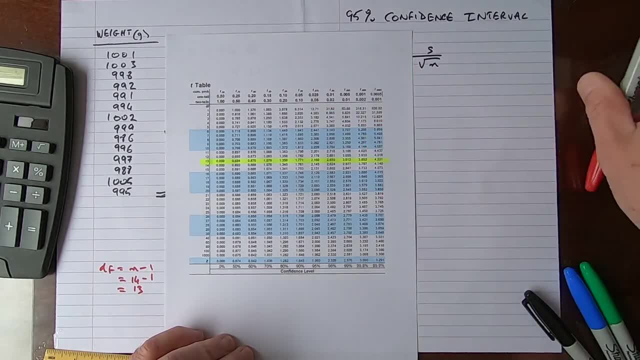 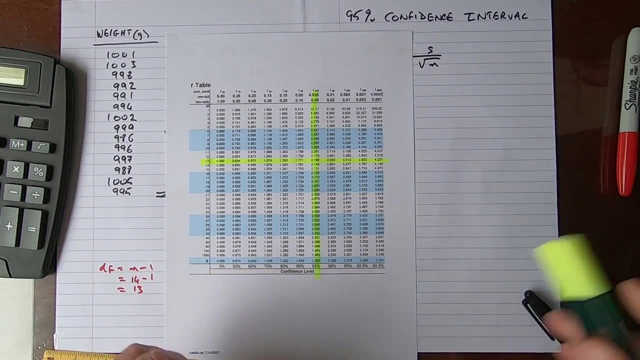 we've got two tails, the value of 0.05, so so somewhere on this column is going to be my t value, and where the two values cross over is the T value I'm going to need. We can see that that is 2.160.. By the way, if you wanted to do a 99% or a different value here, 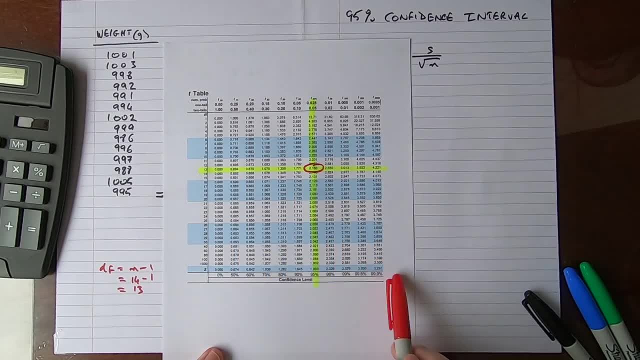 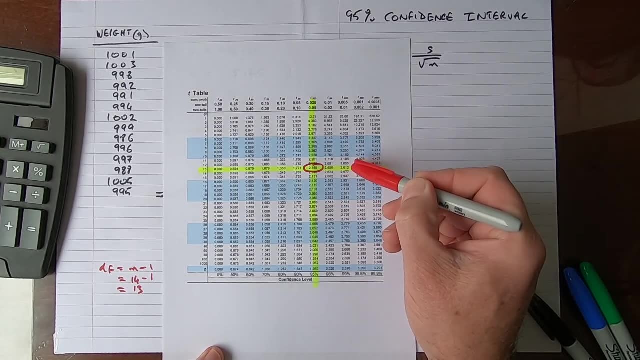 you would have the same degrees of freedom in this sample size but you can see here it would move over. so for example, at 99% confidence interval my T value is going to be 3.012. but we're going to stick with 95% confidence for. 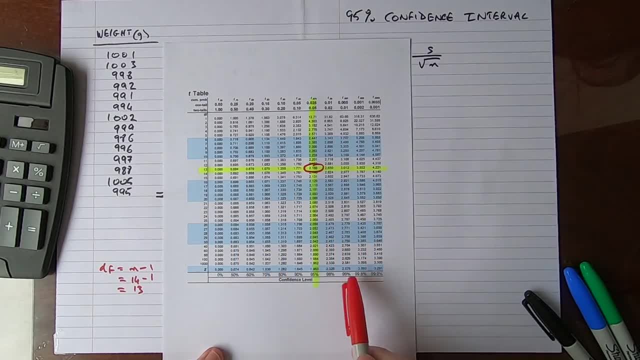 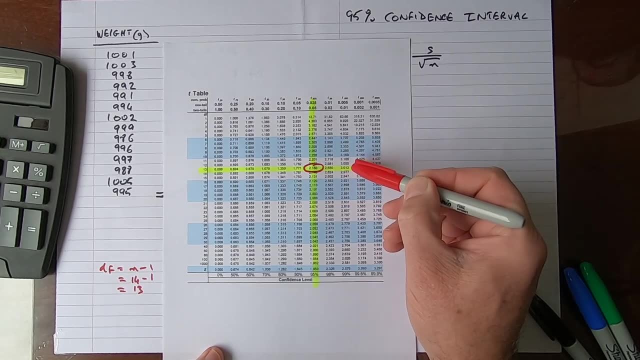 By the way, if you wanted to do a 99% or a different value here, you would have the same degrees of freedom in this sampleed science, but you can see, here it would move over. So for example, at 99% confidence interval my t value is going to be 3,012.. But we're going to stick with 95% confidence for 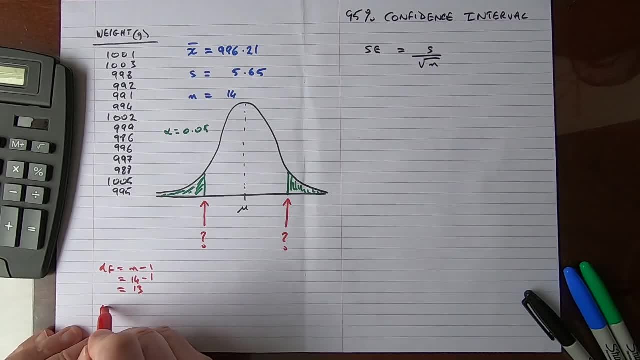 the moment. So my t value course, with proving in time, 0.45- coincidence- is going to mean 0.192.. You see, over here is not 5,000, and the value of 0.192, as we noted earlier, if I move over close here, this value is going to be��다. but that seems to mean that at 99% confidence that you're going to need. 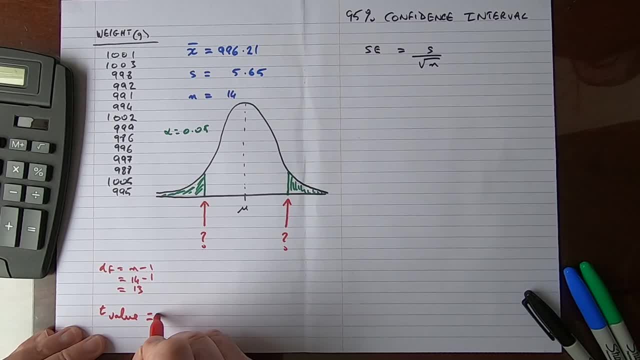 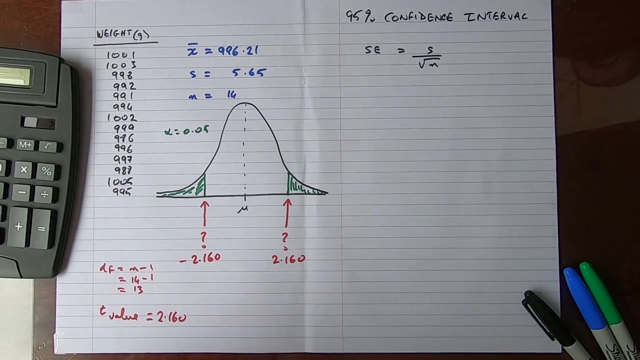 value is equal to 2.160. so that's these values. here is 2.160 and minus 2.160 here on the left tail. now that value is going to become important in a moment. next we need to be able to work out the standard error. so the standard error formula, our standard error of the mean, is a straightforward. 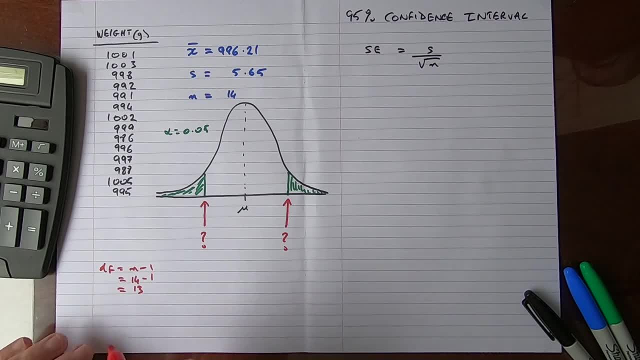 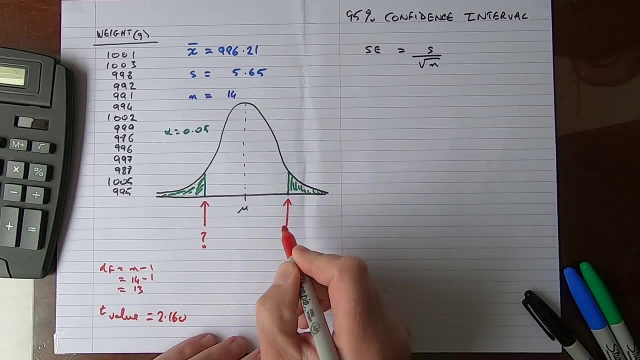 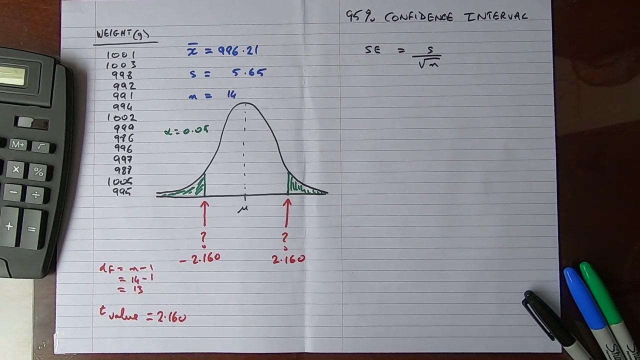 the moment. So my T value, my T value, is equal to at 2.160. so that's these values: here is 2.160 and minus 2.160 here at the left tail. Now that values going to become important in a moment. Next, we need to be able to work out the 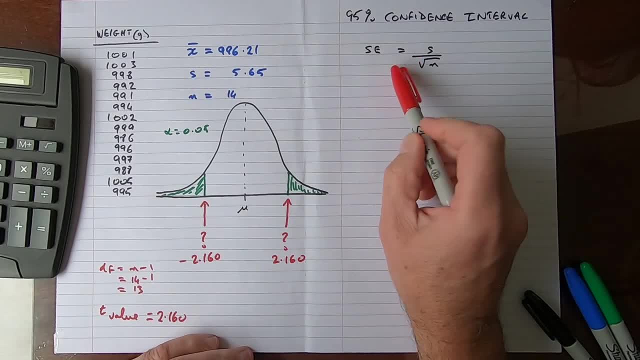 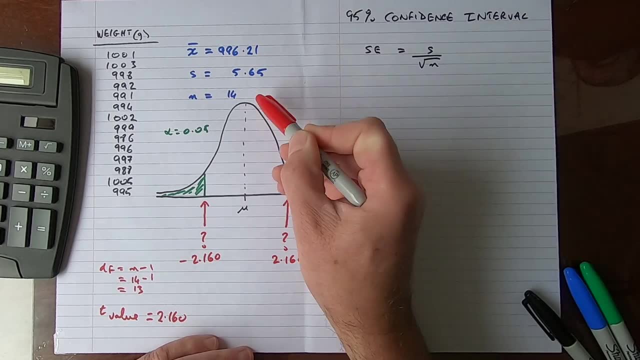 standard error. So the standard error formula, or standard error of the mean, is a straightforward formula. We're using the sample standard deviation here s and divided it by 1. by the square root of n, which in our case is 14.. 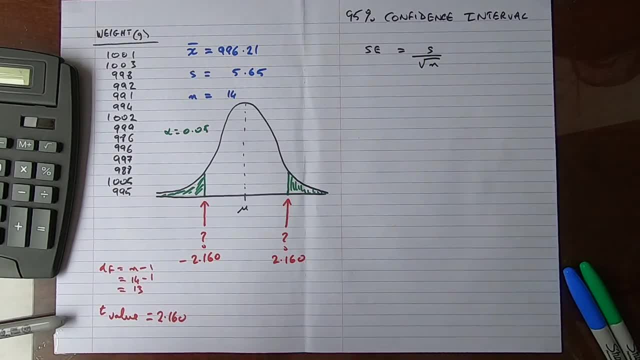 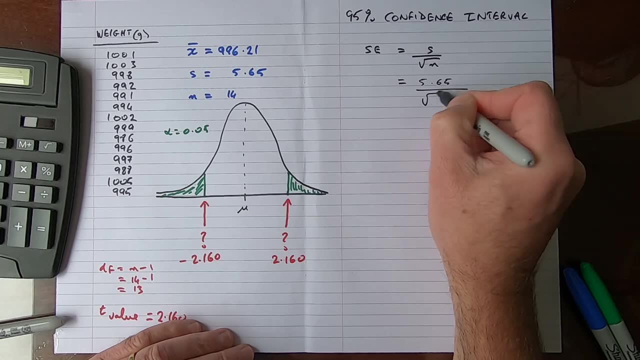 So we have the two values here, So let's go ahead and work this out. So that is equal to a standard deviation of 5.65 divided by the square root of 14.. Let me get my calculator out and work that out. 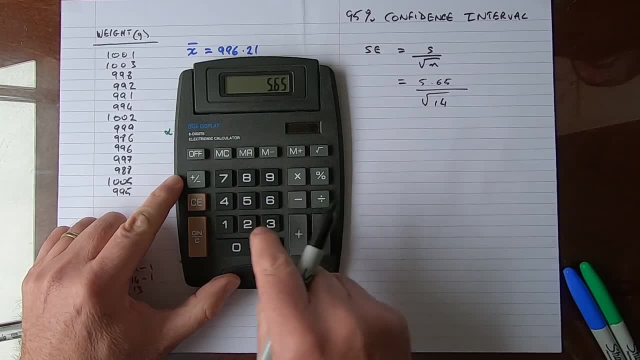 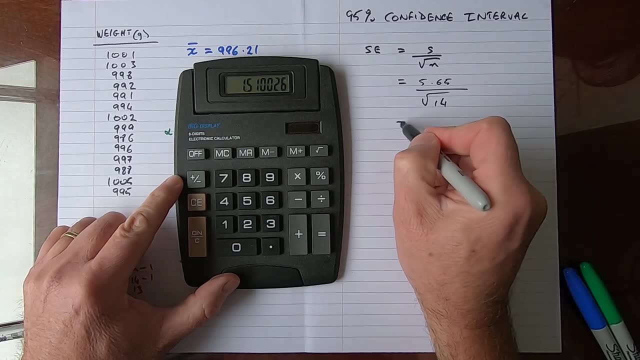 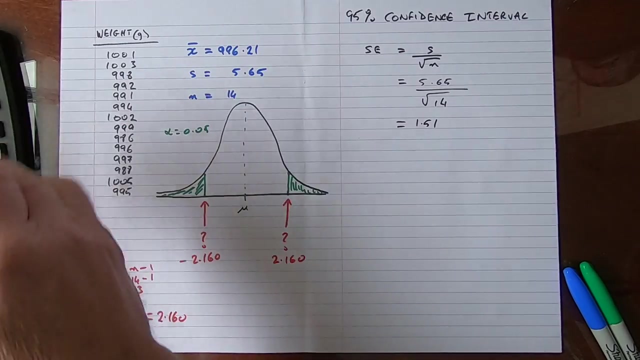 So 5.65 divided by, I'll put in 14 and use the square root symbol to get that and then press equals And that will give me a standard error of 1.51.. I'll use two decimal places there. So now we've got the standard error. 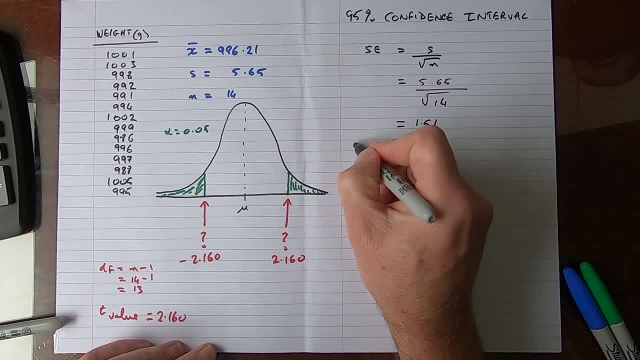 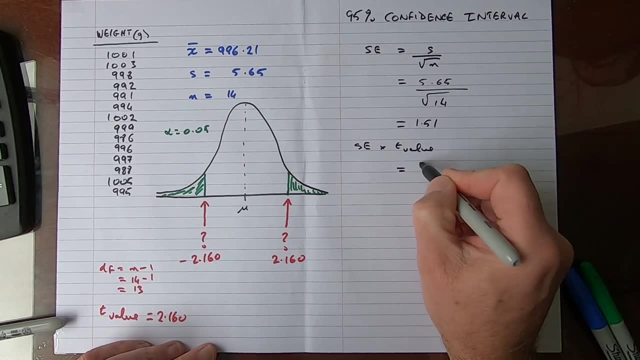 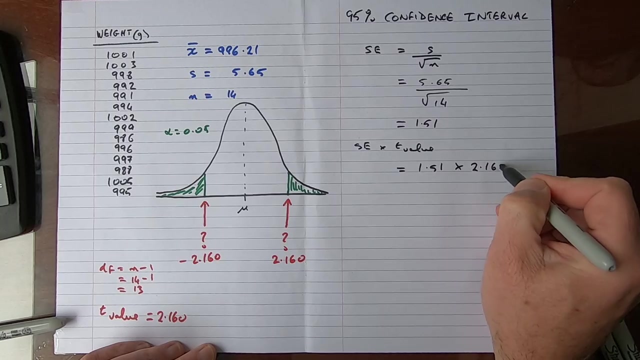 and our next job then is to multiply our standard error. So we want to multiply our standard error multiplied by our T value. So that is equal to 1.51 from here multiplied by 2.160.. So let's work that out. 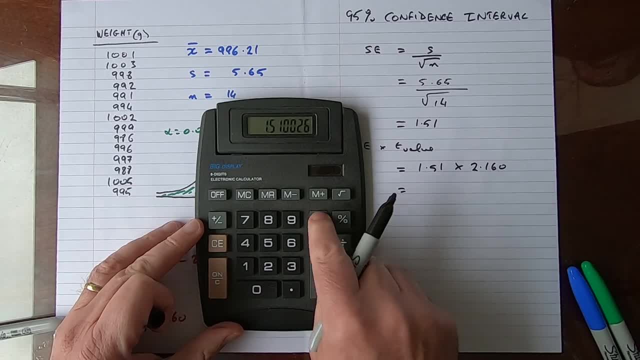 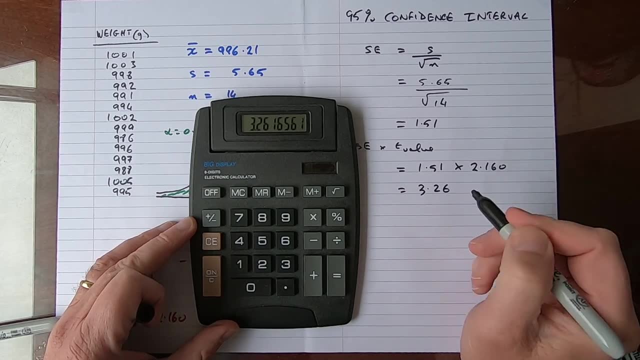 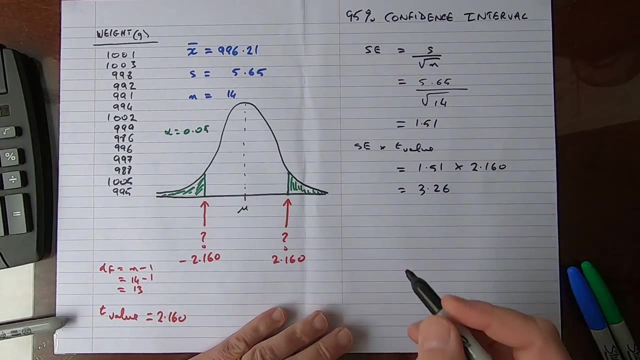 So we have the 1.51 still in our calculator. multiply that by 2.16, that is equal to 3.26.. So now we have the value that we need to estimate our upper value and our lower value for the confidence interval. 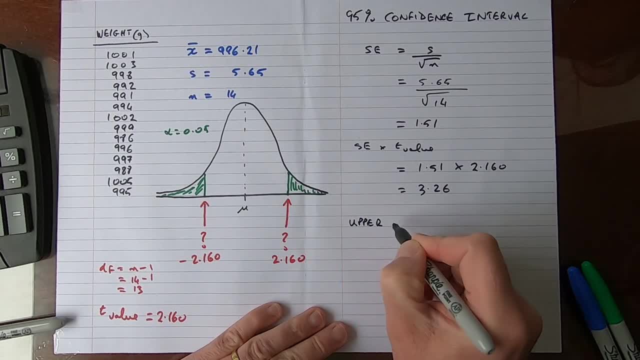 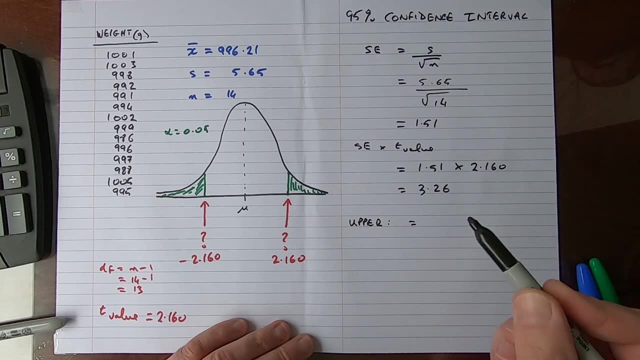 So let me put in the upper one first, And that's going to be equal to my mean 996.21, plus this value that I've just worked out here. So that's going to be 996.21.. So if we look at this, 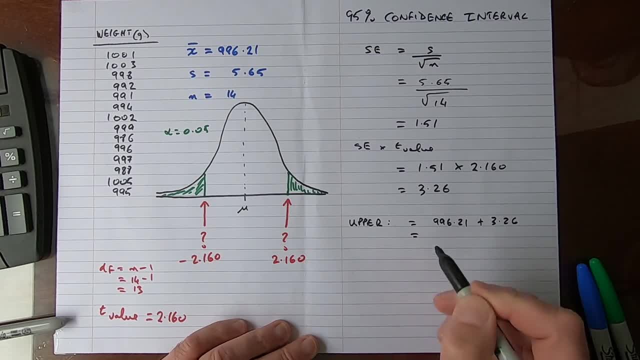 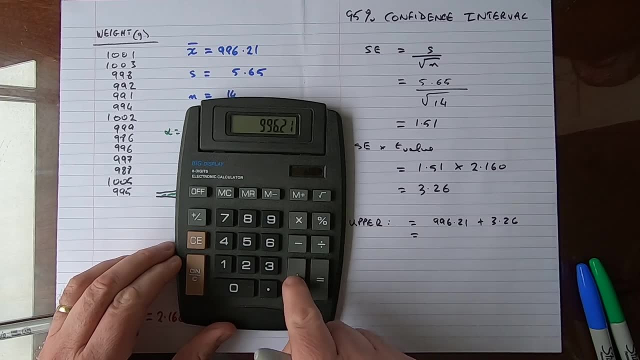 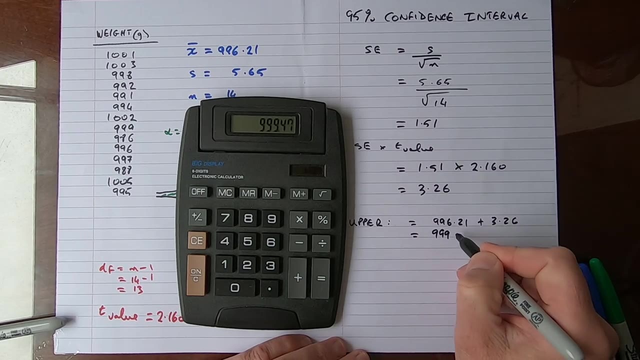 996.21 plus 3.26, and that's going to be equal to. let me work that out with my calculator. So 996.21 plus 3.26 is equal to, so that's 999.47.. And my lower limit. 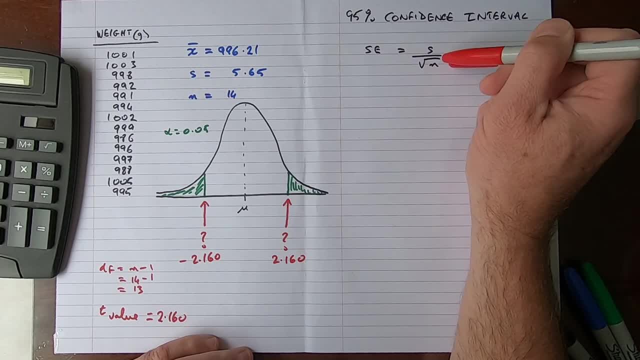 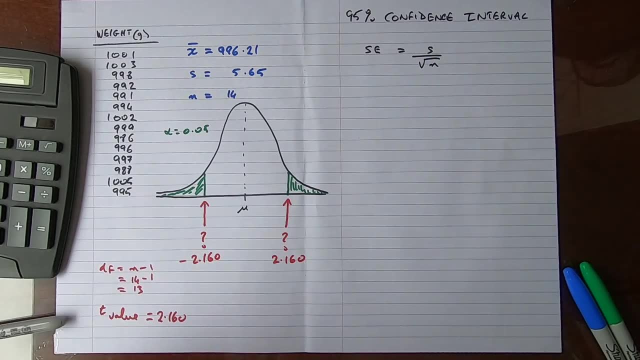 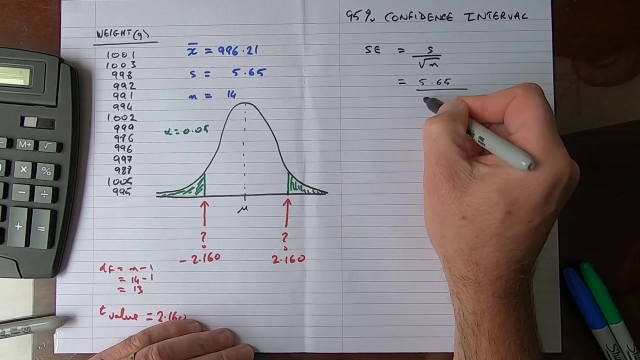 formula. we're using the sample standard deviation here, s and divided it by the square root of n, which in our case is 14, so we have the two values here. so let's go ahead and work this out. so that is equal to a standard deviation of 5.65 divided by the square root of 14. 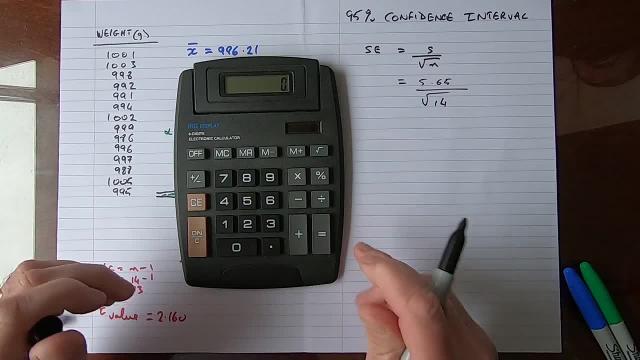 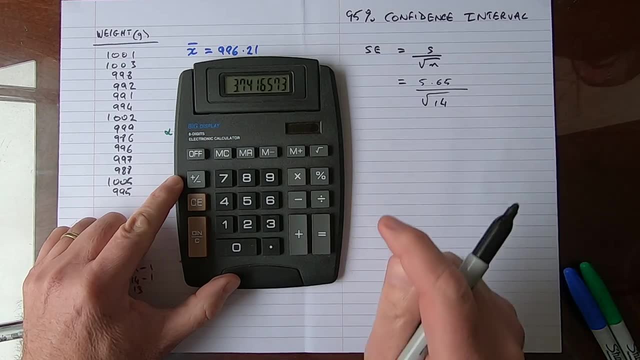 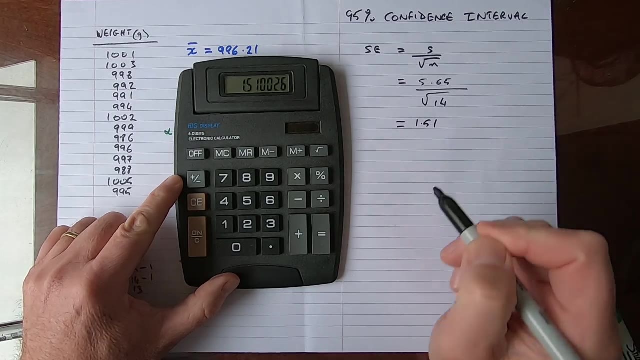 let me get my calculator out and work that out. so 5.65 divided by putting 14 and use the square root symbol to get that, and then press equals, and that will give me a standard error of 1.5 one. I'll use two decimal places there. so now we've got the standard error and our next job. 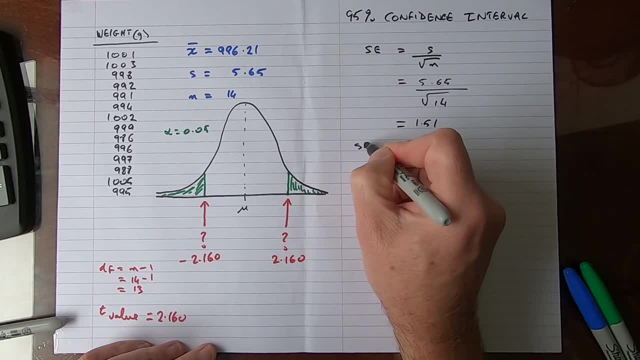 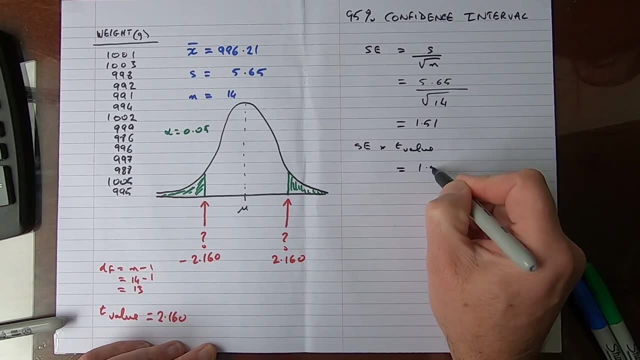 then is is to multiply our standard error. so we want to multiply our standard error multiplied by our t value, so that is equal to 1.51 from here multiplied by 2.160. so let's work that out, so we have the 1.51 still in our calculator. multiply that by 2.160. 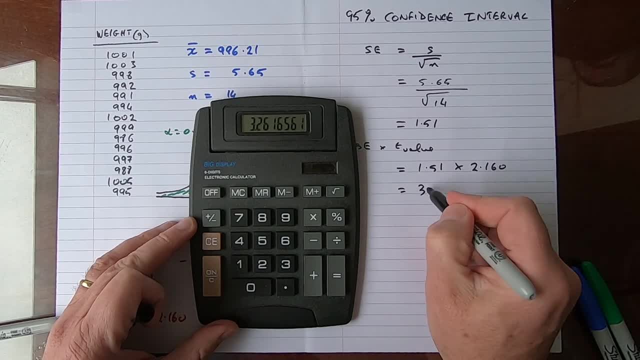 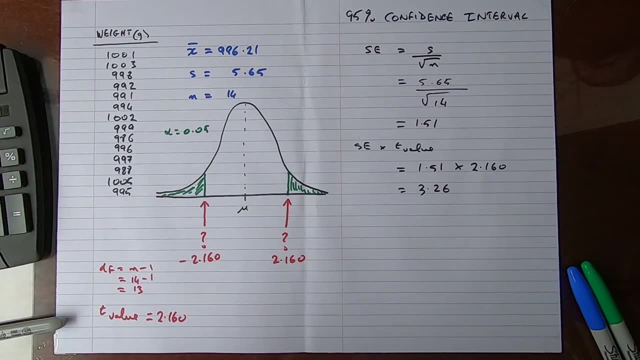 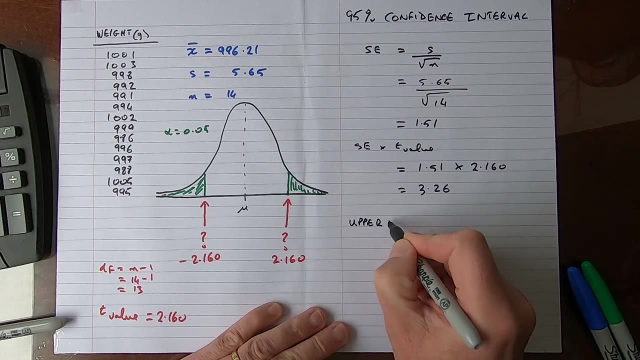 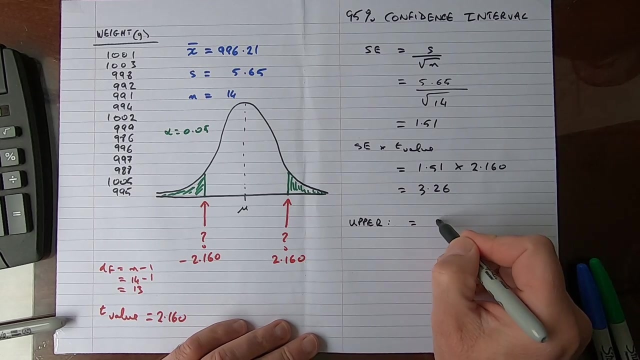 that is equal to 3.26. so now we have the value that we need to estimate our upper value and our lower value for the confidence interval. so let me put in the upper one first, and that's going to be equal to my mean 996.21, plus this value that I've just worked out here. so that's going. 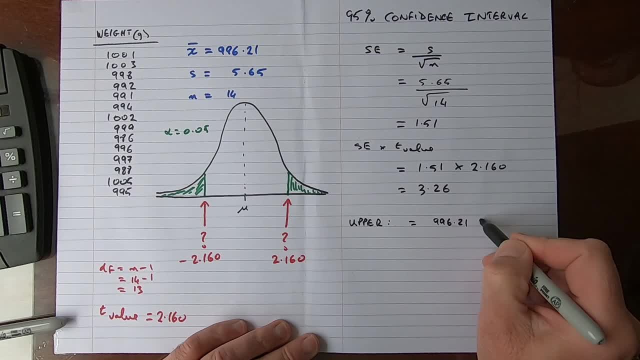 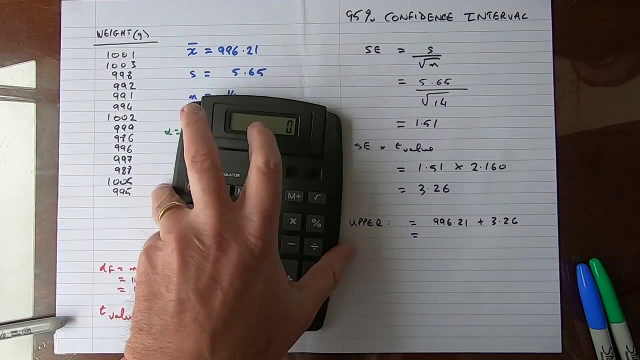 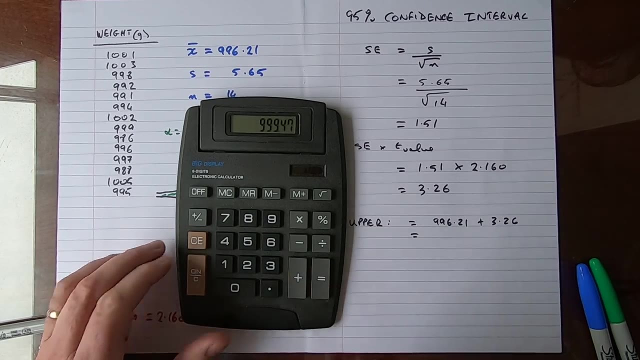 to be nine, nine, six point two, one plus three point two, six, and that's going to be equal to. let me work that out, my calculator. so nine, nine, six point two, one plus three point two, six is equal to: so that's 99, nine nine nine point four, seven, and my lower. 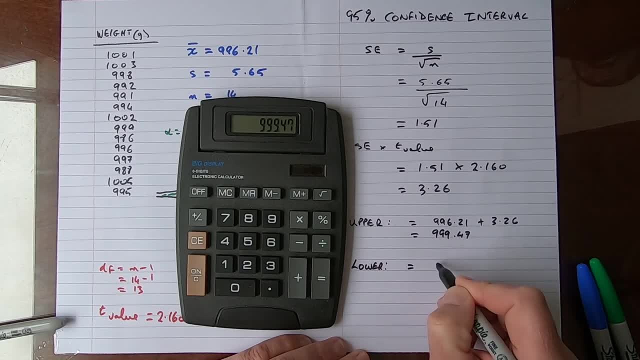 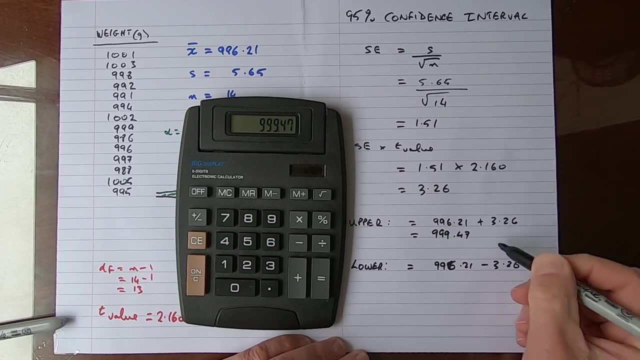 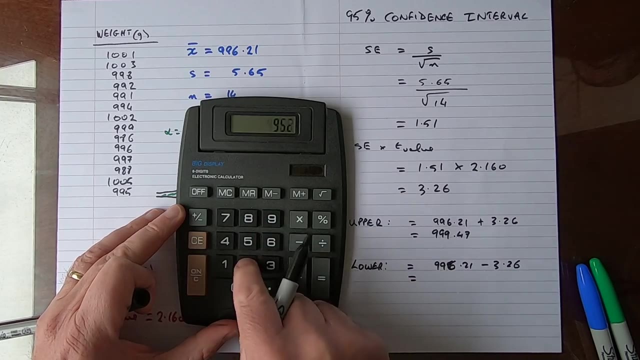 limit for the confidence interval is equal to the same mean value. again, nine, nine, nine, six point two, one minus three point two, six, the same value we worked out here, and that is equal to- let me work that out- nine, nine, six point two, one minus, this time, three.